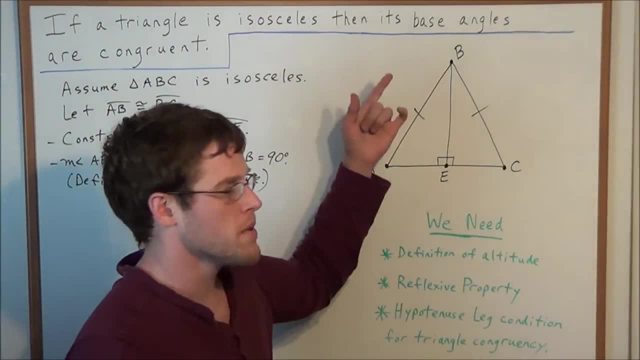 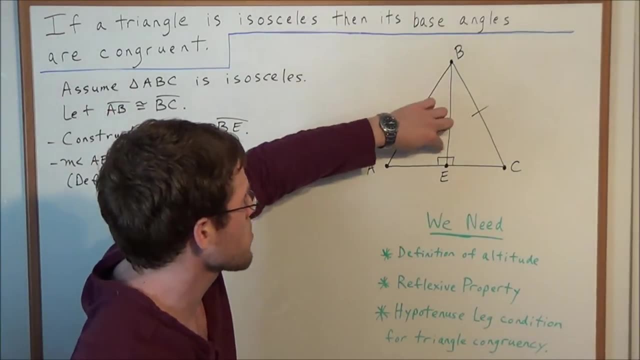 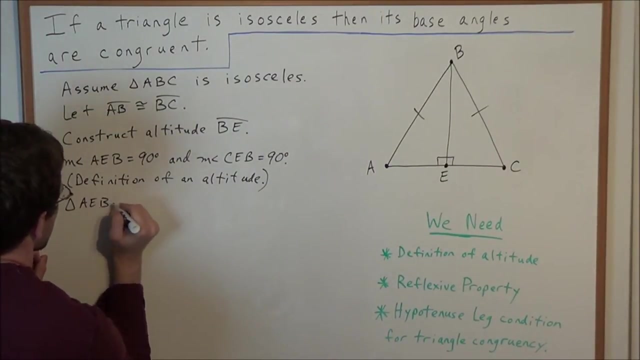 So now from here we need to state, even though it may be obvious: when we construct this altitude, we create two right triangles, Because these two triangles here both contain 90 degree angles. this allows us to say that triangle AEB and triangle CEB are proportional. 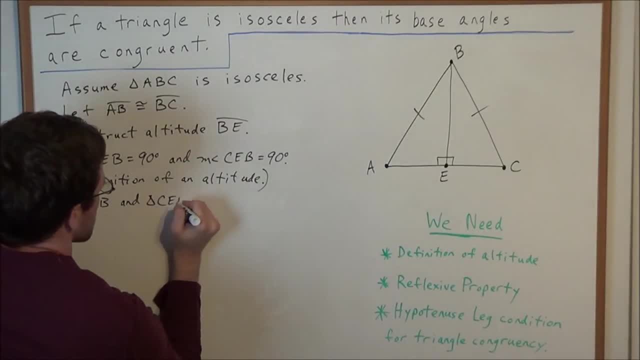 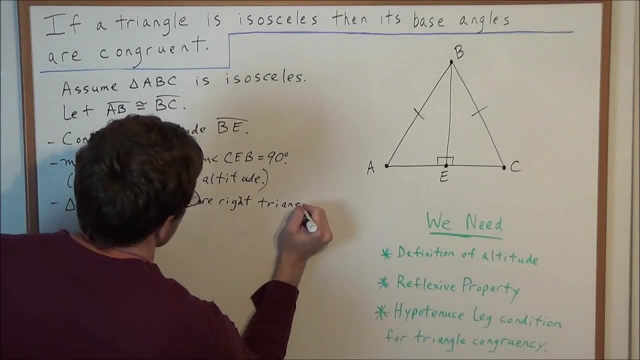 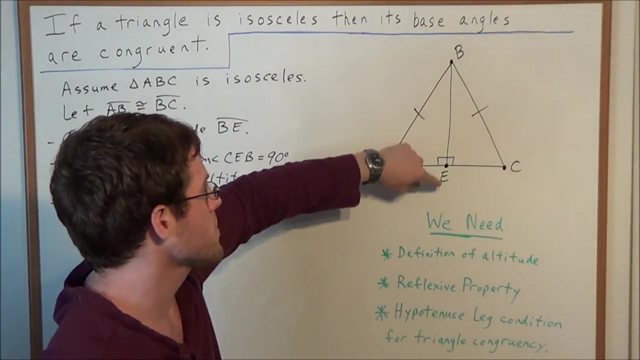 So this is the right angle. Let's say we have the following: Every triangle, Every triangle, Every triangle are right triangles and why they both contain right angles. okay, so now the next step. we could say that line segment BE is congruent to itself. this seems. 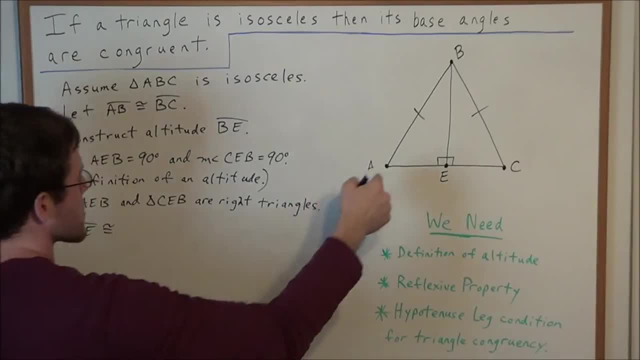 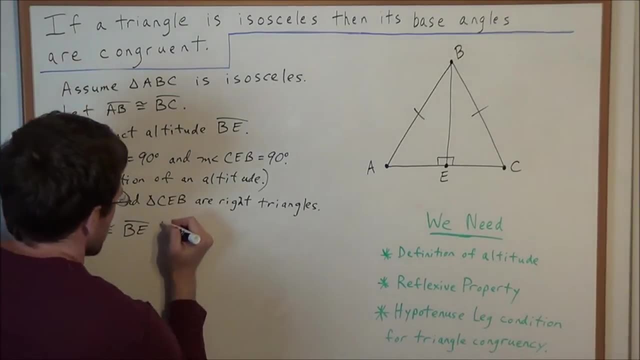 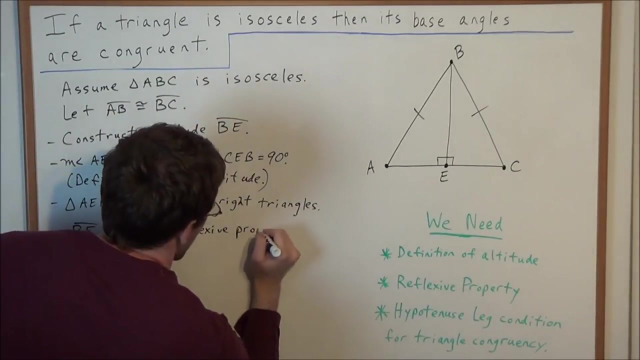 really obvious, but this is critical for proving that these two triangles are congruent. so we say that line segment BE is congruent to the line segment BE by the reflexive property of equality. so reflexive property which, if we think about the reflexive property, all it states is that some line segment or some. 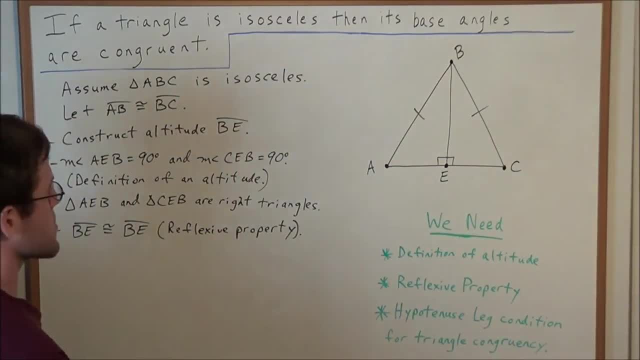 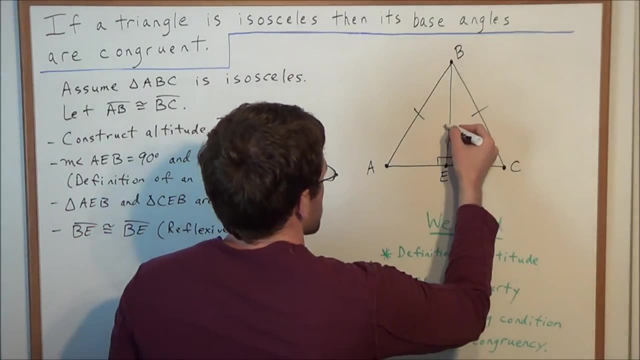 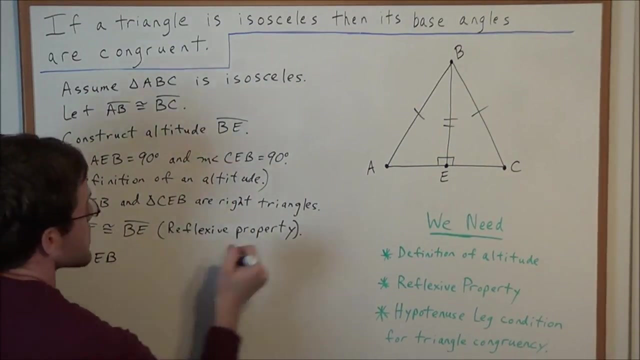 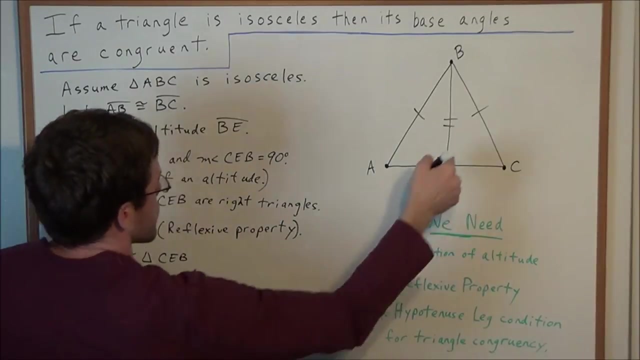 figure is congruent to itself. but now, what does this allow us to say? well, we have two right triangles and they share the same hypotenuse and they share the same leg. so this allows us to say that triangle AEB, which is here, is congruent to triangle CEB, which is the right triangle right. 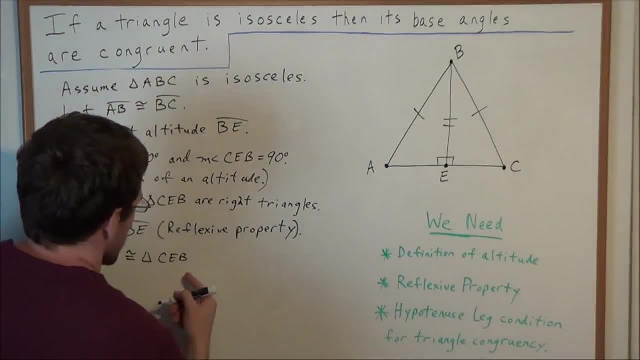 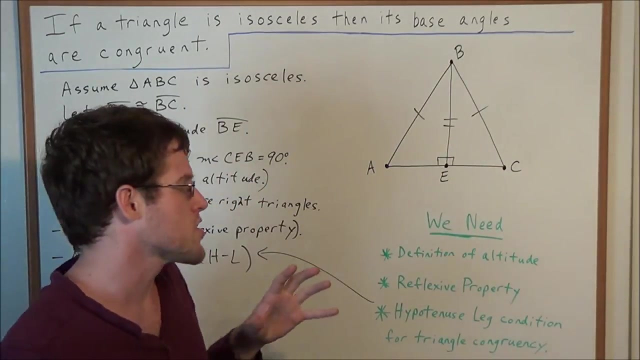 next to it. So these two triangles are congruent. and the reasoning for this I'll just abbreviate: the hypotenuse leg condition for triangle congruency. So when we're doing triangle proofs, when we have a right triangle, it's a special. 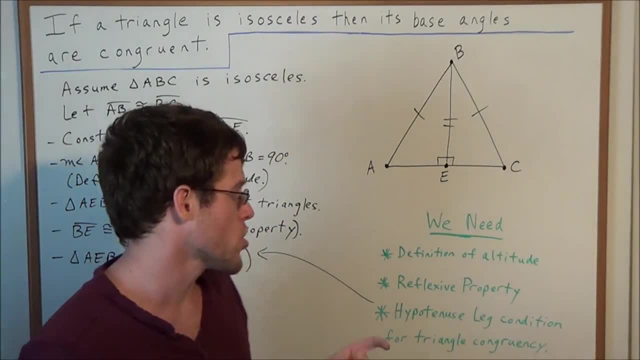 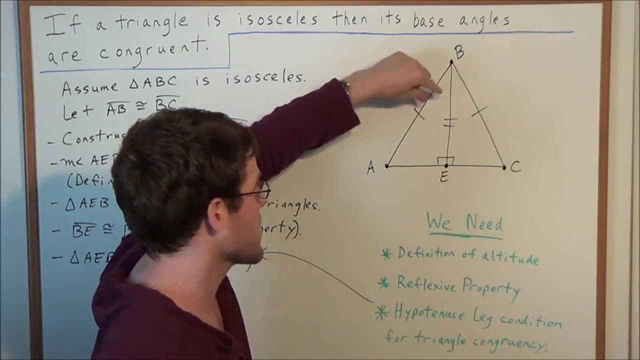 case where we don't need to use the side-side-side condition for triangle congruency, It's sufficient enough to say that if they share a common leg and a common hypotenuse, then those two right triangles are congruent. And the quick explanation for why is because if we used a Pythagorean theorem we could: 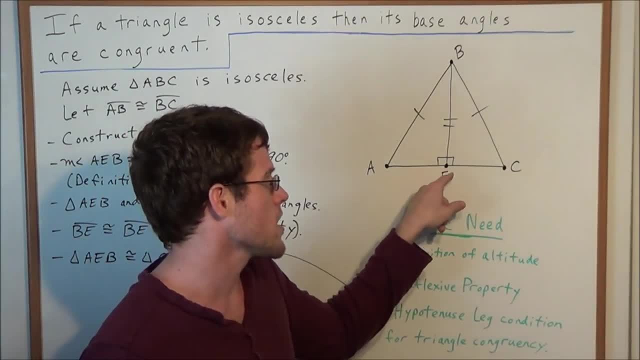 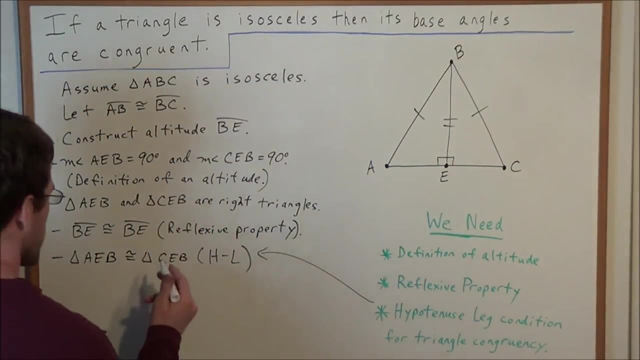 reason that this side and this side that line, segment AE, is congruent to EC And that would give us the side-side-side condition for triangle congruency. So now that we know these two triangles are congruent, we could say that angle.